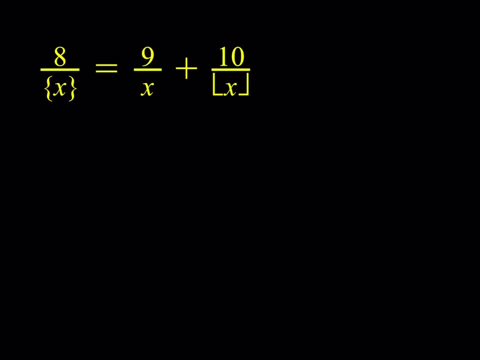 Hello everyone, In this video we're going to be solving a floor value equation. If you like this video, please comment, like and subscribe, and hit the bell button for notifications and let's get started. So we have this equation where 8 is divided by the fractional part of x. 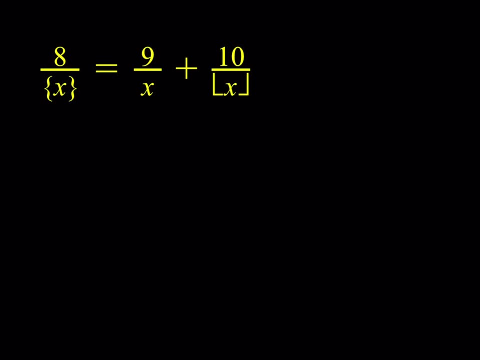 which I'm going to define in a little bit. That is equal to 9 over x plus 10 divided by the floor value of x. So we're going to solve for x values here and let's go ahead and start with the definition of floor value and the fractional part of x. Okay, so how is floor value defined? 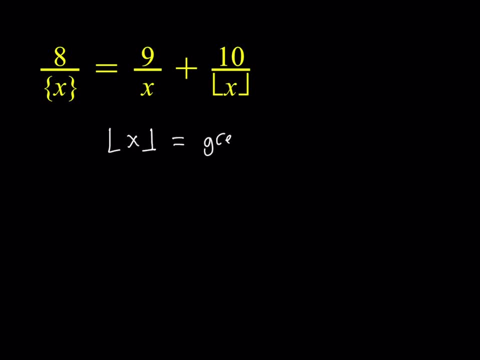 Well, the floor value of x is basically the greatest integer. It's also called the greatest integer function less than or equal to x. So basically it's it's kind of like we could probably define it as rounding the number down to the nearest integer, but that's not necessarily. 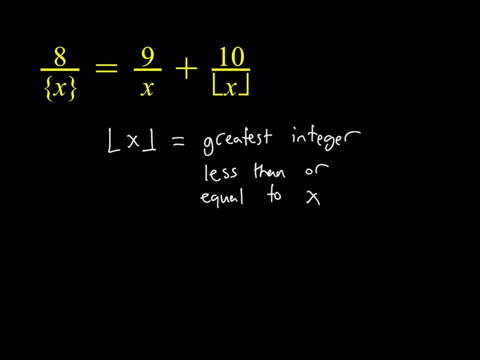 the well, if you say rounding down, it's always true because we're always rounding down. Okay, that's why it needs to be less than or equal to x. So, for example, if you're looking at the floor value of pi, that's going to be 3 because 3.14, but if you look at the negative pi- that's kind of interesting- it's not going to. 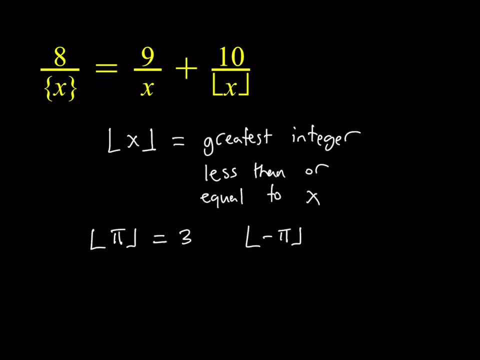 be negative. 3 because negative pi is negative 3.1, something, and that is going to be negative. 4 because the number, the floor value, is always less than or equal to x. So we can safely say that the floor value of x is always less than or equal to x. Now comparing these two numbers, the floor value, 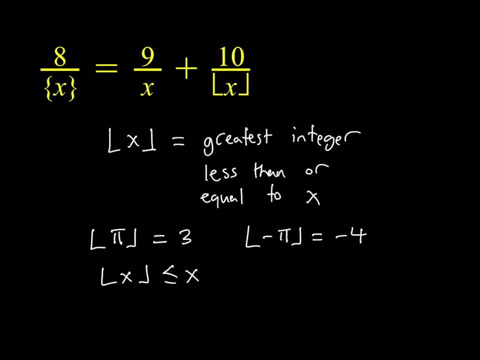 of x and the x itself. we're kind of looking at the difference here. So, for example, if you consider pi 3.14 and then the floor value of pi is 3, so the difference is 0.14.. So the fractional part of x is basically. 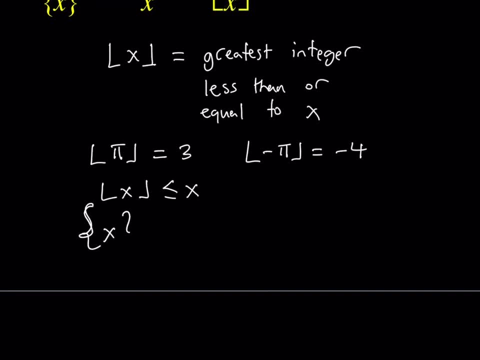 then defined as the fractional part of x, which we use the braces for. that is defined as x minus the floor value of x. Okay, so if you take away the floor value of a number from itself, you end up with the fractional part of x. So if you take away the floor value of a number from itself, you end up with the fractional part of x. 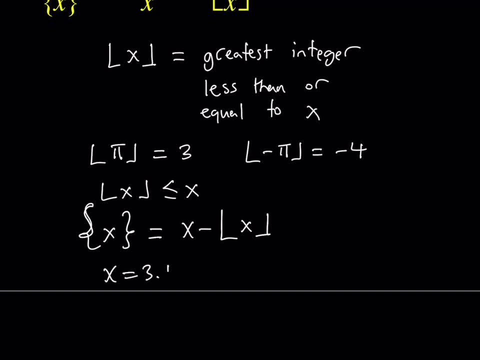 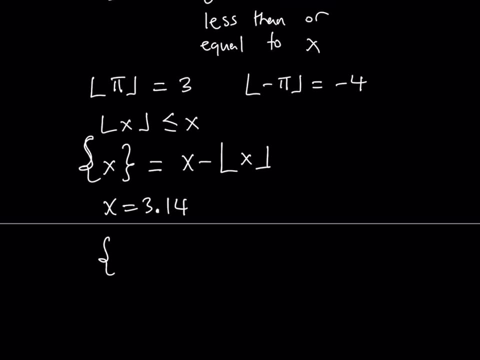 So in this case, for example, suppose x is equal to 3.14, and this is obviously not exactly pi but just an approximation, and in this case the- you know the fractional part of 3.14 is just going to equal 3.14 minus the floor value of 3.14, which is 3, and it's going to be 0.14.. Okay, that's basically. 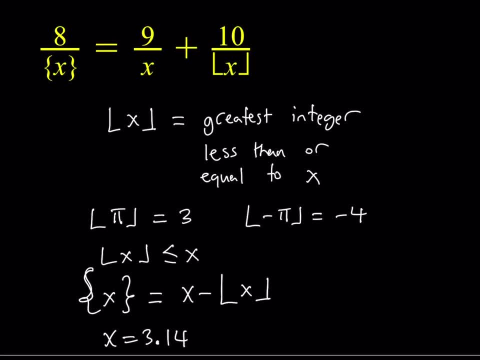 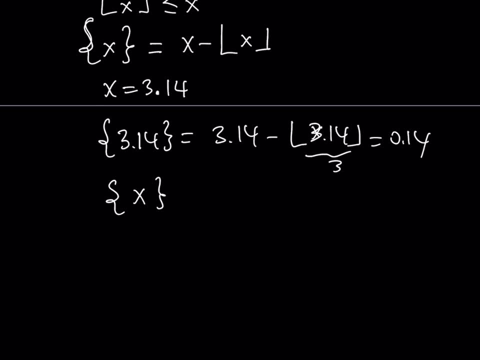 how we define the fractional part of x. Now let's go ahead and take a look at our equation. So one of the things that's significant about the floor value and the fractional part of x is that the obviously so. for example, if you think about it like if x is an 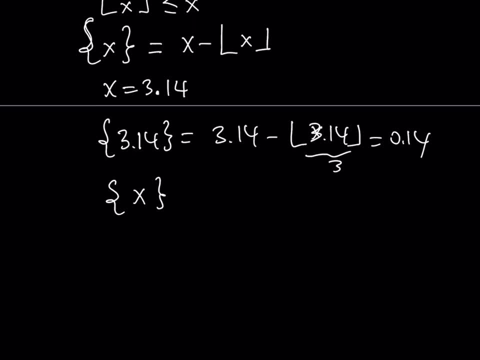 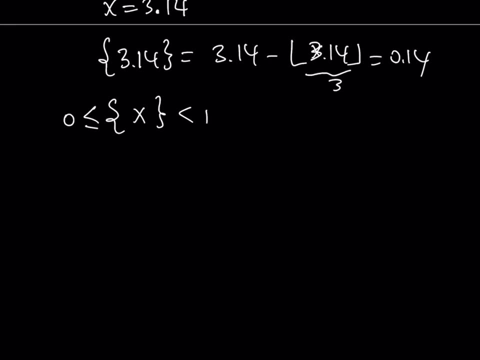 integer, then it's going to be 0. So basically you're looking at a value between 0 and 1. here 0 is inclusive. Okay. so looking at from that perspective, our equation, 8 divided by the fractional part of x is equal to 9 over x plus 10 over floor value of x. Here you notice that. 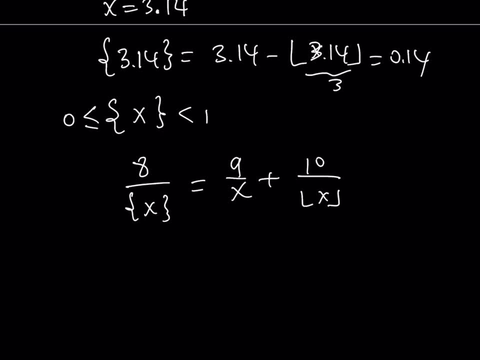 since this number is, obviously it can't be 0 in this case. So we're going to take a look at the this case, right? Since this number is less than 1, when you divide 8 by that, you're basically going to be getting something greater than 8, right? So we can safely say that 8 divided by the fractional 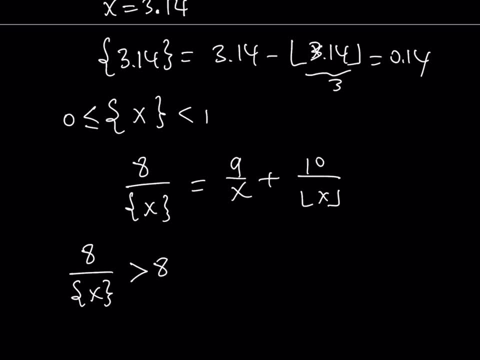 part of x is greater than 8.. Okay, which implies that the right hand side is also greater than 8.. So let's take a look at it from that perspective, and this should also be greater than 8.. So that gives us some bounds. That's what we're going to work with here, because with floor value equations, 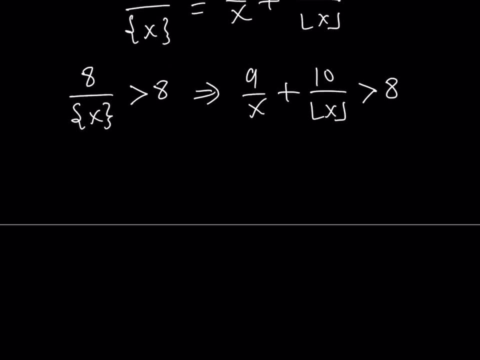 play an important role. Okay now, if you look at this equation from that inequality perspective, notice that, for example, if x is equal to 3, what are you going to get? If x is equal to 3, then we're going to be getting 9 divided by 3 plus 10 divided by. 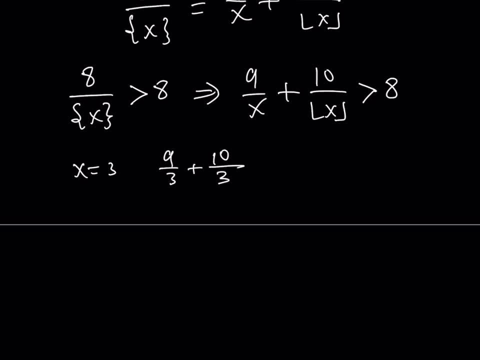 3, and this is going to give you 3 plus 3.3, something repeating, and the sum is not going to be greater than 8.. Make sense. So for x equals 3. this sum, this inequality, is not satisfied. What about anything greater than 3?? Obviously, as x is. 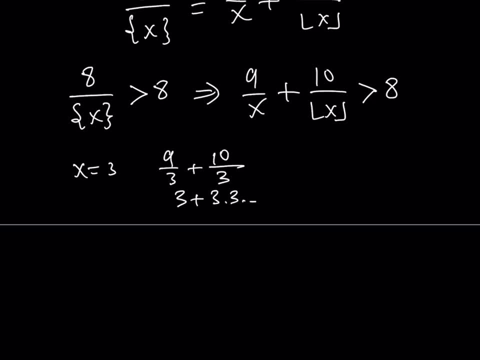 greater than greater. this left hand side is going to be smaller. I'm talking about this left hand side, So it's never going to be greater than 8.. So we can safely say that for x is greater than or equal to 3, there are no solutions. Wow, this is really cool, right? This is nice, because now we 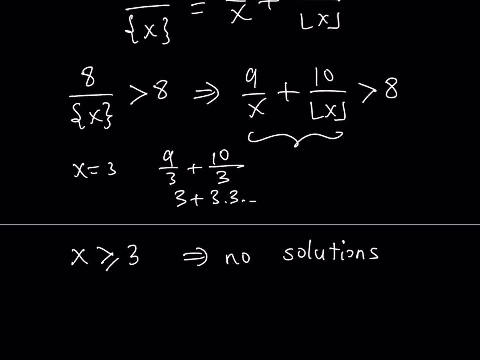 were able to find an upper bound. Well, why is this an upper bound, though, or do we have a lower bound? So let's kind of look at some negative numbers, right, or numbers that are in the range of zero to one, But first of all, what happens if x is negative? Well, if x is going to be negative, then let's take a look. 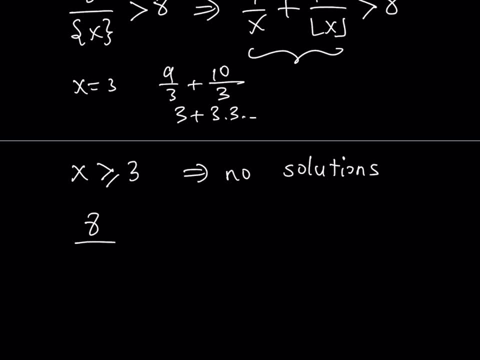 and, by the way, this expression, since x is always the fractional part of x, is always non-negative. this is always going to be greater than zero. obviously right for any, any number. Well, yeah, it's going to be greater than zero. So what is that supposed to mean? 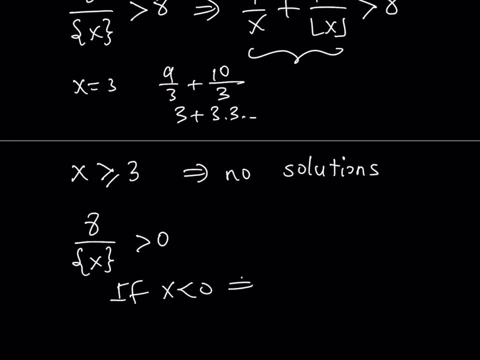 If x is negative, then you'll have 9 over x plus 10 over the floor value of x. This is going to be a negative quantity. but this is impossible. You can't have one side greater than zero, the other side less than zero. So that means that x needs to be greater than or equal to zero. but we already 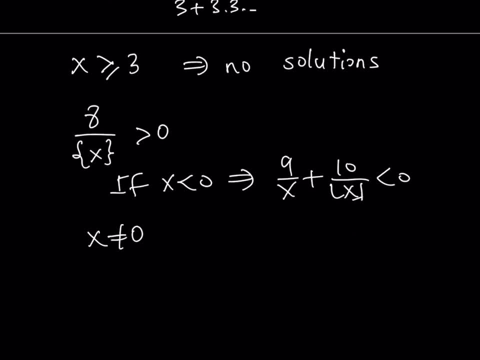 talked about it. x cannot equal zero, which means that x needs to be greater than zero- We know that for sure- And x needs to be less than x needs to be less than three. So we basically have that x needs to be between zero and three non-inclusive. Okay, that's basically what we get. 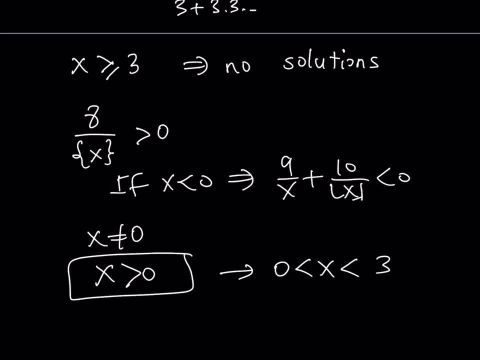 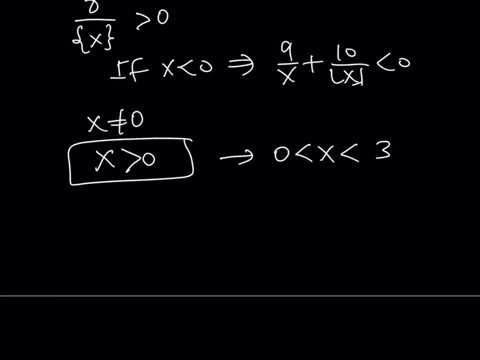 as a result. So we have a lower bound as well as an upper bound, which is really nice, because we're only going to be looking at the intervals, And it makes sense to break down this interval into sub-intervals, such as: what happens, for example, if, if x is between zero and one right? Well, if x is. 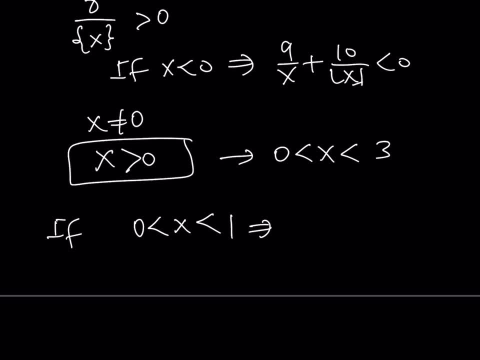 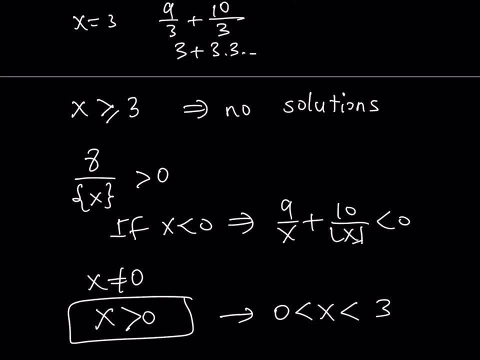 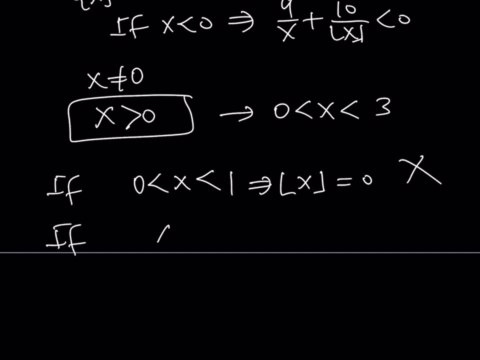 between zero and one, then basically, from here, the floor value of x is going to be zero, right, and that's going to make our expression undefined. So x cannot be between zero and one. this case does not work. What happens if x is between one and two? right, So now we're going to 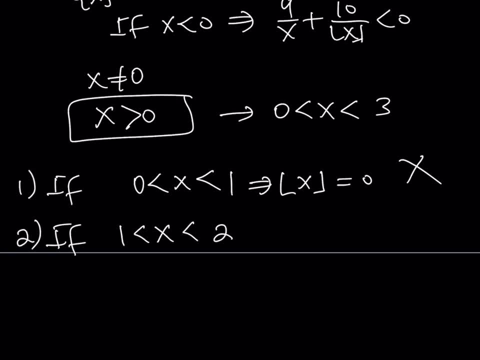 look at the second case and we can number these cases. So we're going to be looking at case by case Case number two: what if x is between one and two? Okay, cool. Now, if x is between one and two, this means that the floor value of x- so you're talking about something like 1.5, 1.2, 1.09, whatever. 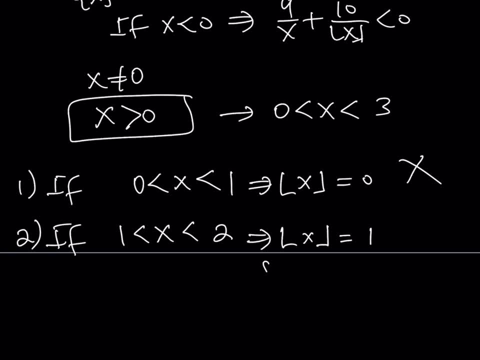 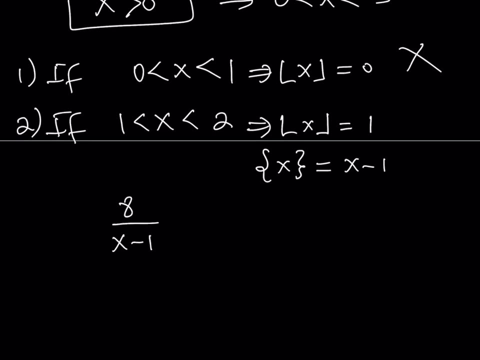 x is going to be 1 because you're rounding it down right And, as you know, the fractional part is just the number itself, x minus the floor value. so it's going to equal x minus one, right, It's easy? So now our equation turns into this: 8 over x minus 1 is equal to 9 over x plus 10.. Great, So now we're. 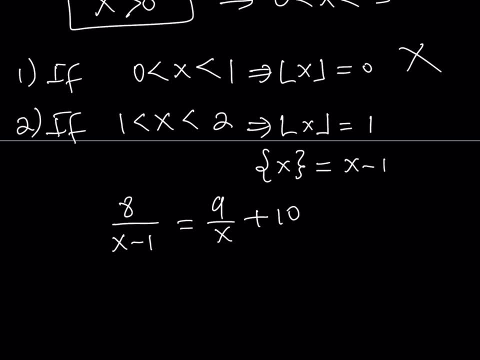 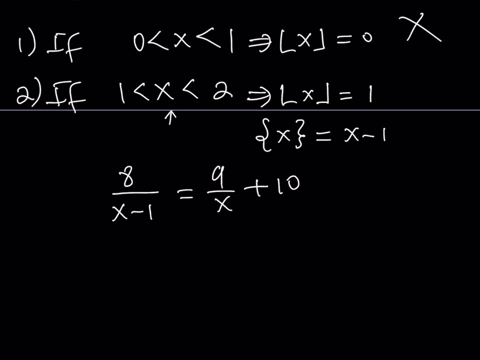 going to solve this equation under this condition that x needs to be between one and two. So let's take a look at this equation from that perspective. Now, how do you solve it? Well, first of all, notice that x cannot be zero, x cannot be one. So that's cool, that's good. Let's go ahead and make a common. 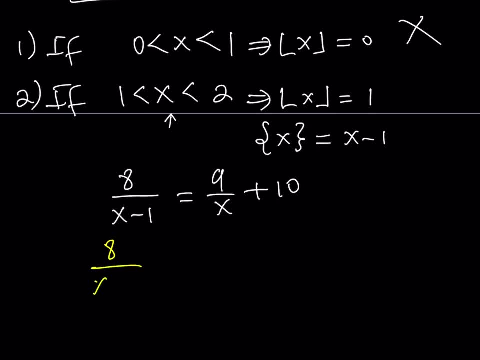 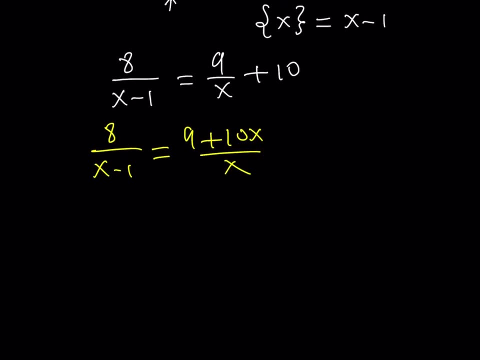 denominator here and let's see what that looks like: 8 over x minus 1 is equal to 9 plus 10 x divided by x, And let's go ahead and cross multiply here and we should be getting something like 8 x is equal to. let's go ahead and distribute the x: 9 x plus 10 x squared, and then I have minus. 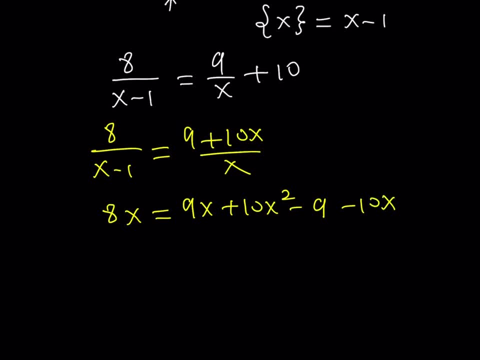 9 minus 10 x. So let's go ahead and put everything on the same side so we get a quadratic. So 8 x subtract from 9 x is going to be 1 x, and then this is going to be negative 10 x right, Negative 10. 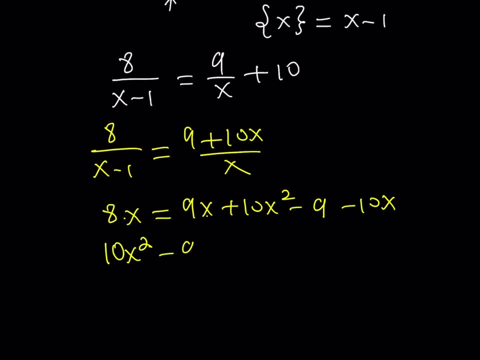 plus 1 is going to be negative 9.. So it's going to be negative 9 x minus 9.. So let's go ahead and solve this equation by using the quadratic formula. I'm not really going to look for factoring, It's. 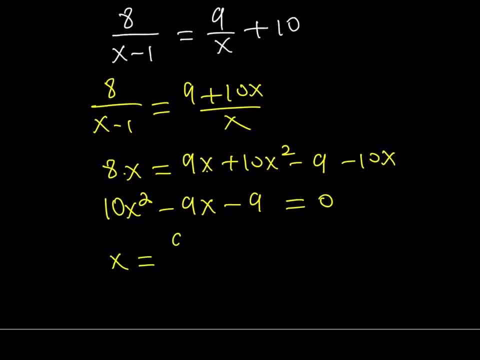 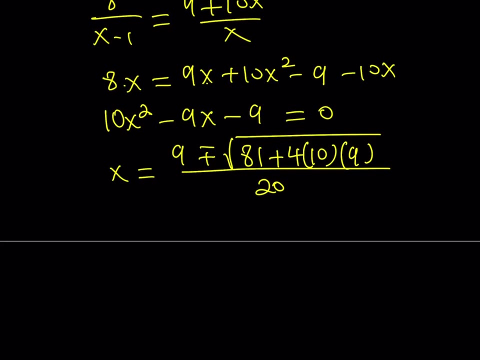 probably factorable. but anyways, let's just use the formula Negative b plus minus the square root of b squared, And that's going to be 81 minus 4 times 10, times negative 9, which is going to make this positive. Okay, let's see if we get a nice quadratic or perfect square from here. Let's see. Okay, so, 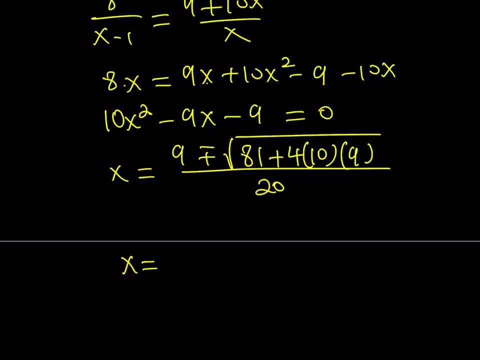 obviously 9 is factorable. We could probably pull that out. If we pull out a 9, that's going to be 9 plus 40, which is 49.. That's cool, because now the square root of that expression is going to be: 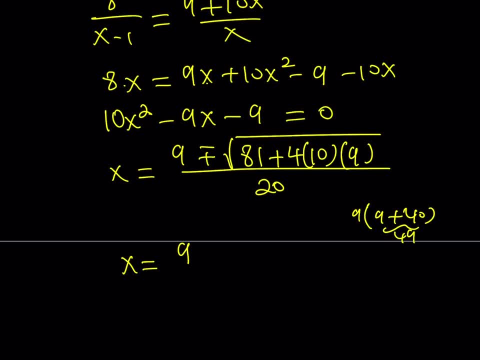 7 times 3, which is 21.. So that was. that was probably 441, which is 21.. So that's going to be 81 minus 4 times 10, times negative 9, which is 49.. That's cool because 21 squared, Anyways. so this is what we get. Obviously, 9 minus 21 is going to give us a. 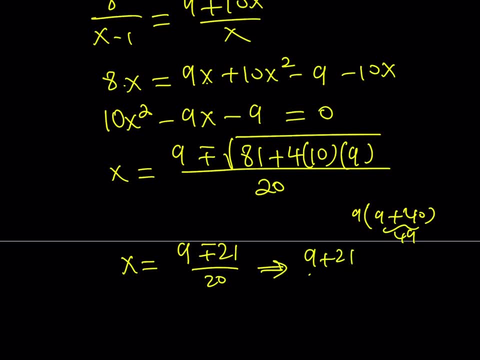 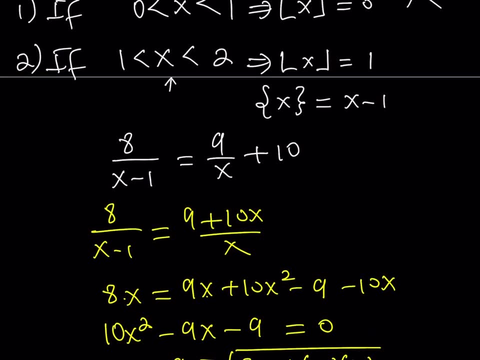 negative answer. We don't want that. So we want 9 plus 21 divided by 20, and that should be 3 halves. Now does 3 halves satisfy our initial condition that x needs to be between 1 and 2?? Yes, it does. 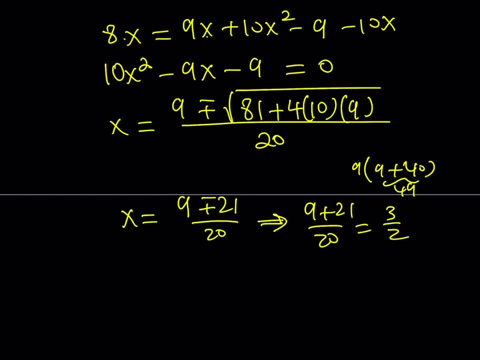 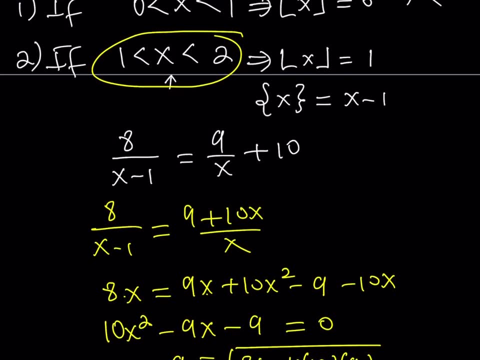 Therefore, we'll accept it. So x equals 3 halves is going to be a valid solution. Okay, now we're going to look at the second case scenario, which is x is between 2 and 3.. So we're going to look at 2 and 3.. Okay, let's take a look at that one. That's going to be condition number 3 or case number 3. 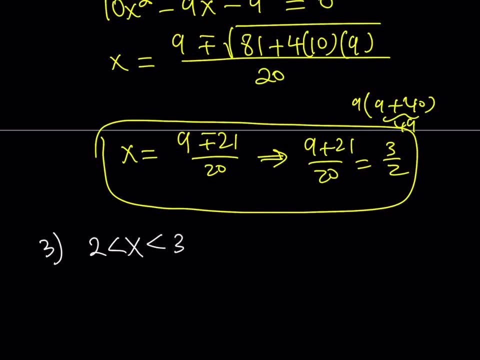 rather, x is between 2 and 3.. Now remember, our original equation was: 8 over fractional part of x is equal to 9 over x plus 10 over floor value of x. So if x is between 2 and 3, its floor value is: 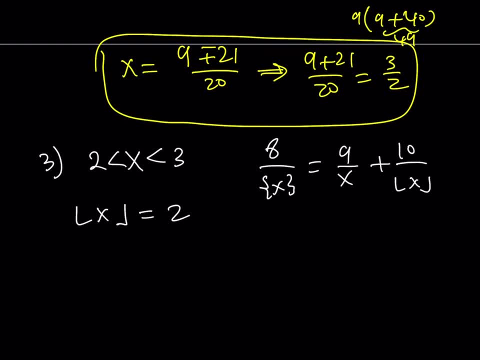 going to be 2, because it's going to be 2 point, something right, less than 3.. And its fractional part, as you know, is going to be x minus floor value of x, Which is going to equal x minus 2.. So we get a different expression every time if we know where x 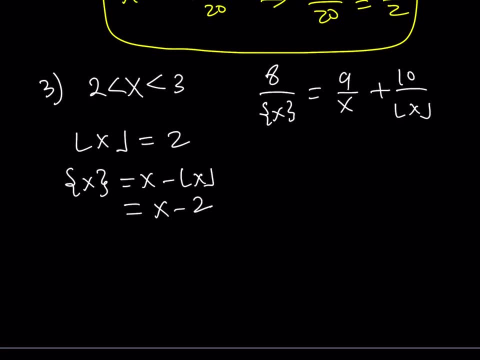 lies. Okay, cool, Now let's go ahead and do the replacements. 8 over x minus 2 is equal to 9 over x plus 10 over floor value of x, which is equal to 2.. So we're able to basically here get a. 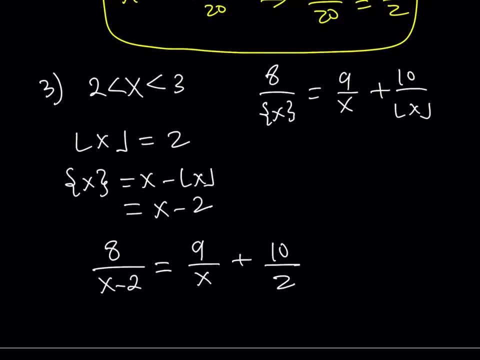 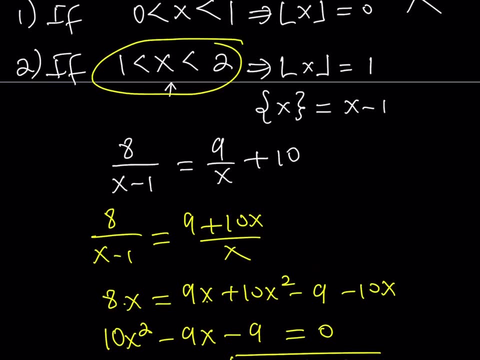 what's it called? get a numerical value for floor value of x, because x lies in a certain interval, And we were able to do that here as well, because 10 divided by 1 is equal to 10.. Make sense, Okay, cool. Now this. 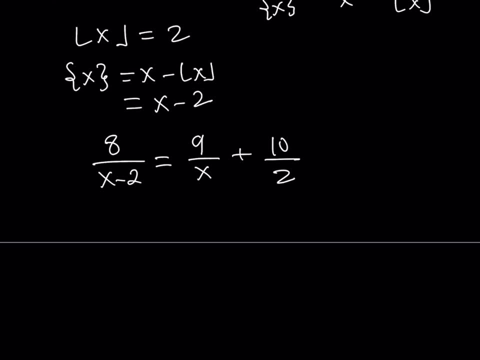 is going to be 5, or we can just make a common denominator without simplifying, And that's going to look like: 8 over x minus 2 is equal to 9 times 2 is equal to 18 plus 10x divided by 2x, which is: 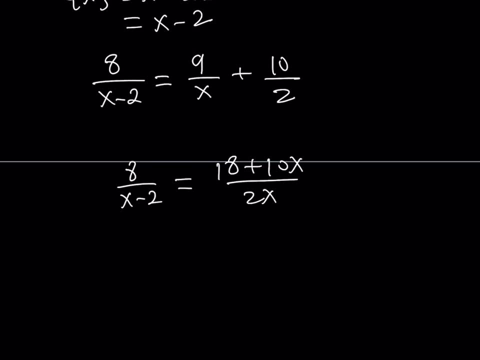 obviously can be simplified later, but that's okay, This is going to give us. let's see: should I divide by 2?? Okay, fine, let's do it. 9 plus 5x divided by x and then 8 times x is equal to. let's go and distribute x first, 9x plus 5x squared, and distribute to negative 2. 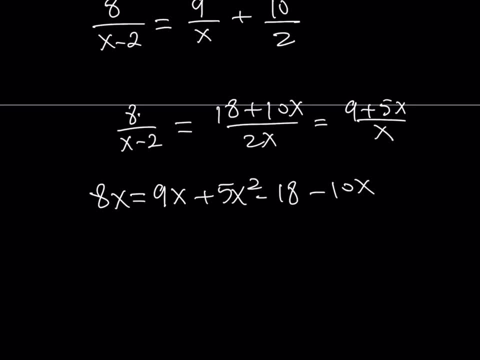 negative: 18 minus 10x. Okay, and then let's put everything on the same side, like before: 5x squared. this is going to bring a positive x again, so it's going to be negative. 9x minus 18 is equal to 0.. You got to remember that x is between 2 and 3 in this case. So let's see if. 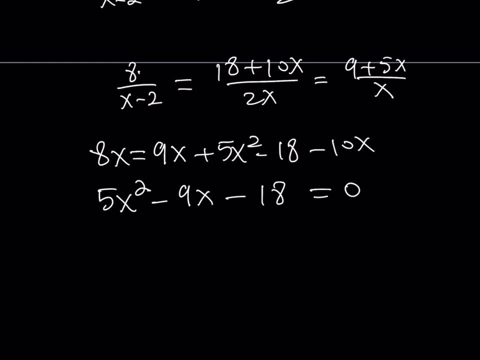 we get any any solutions from here, And when we solve this using the quadratic formula, it should be negative b, which is 9 plus minus the square root of b squared minus 4ac. Obviously that's going to be a positive sign and we're going to get this Again. 9 seems to be a common factor, so I can. 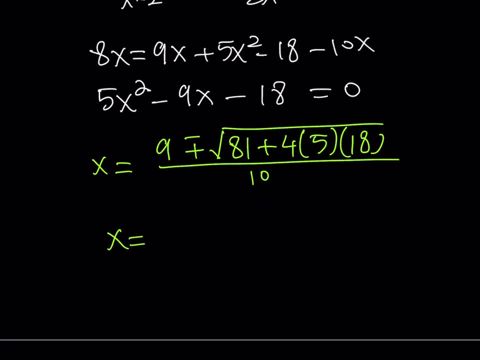 pull it out, Let's see what that gives us. And if I pull out a 9 here, I should be getting 9 plus, so I should. I'll get a 2 here. 4 times 5 is 20.. 20 times 2 is 40. So I'm getting 49 again. So that's. 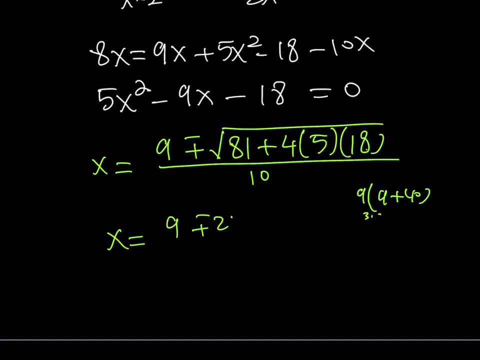 going to be 3 times 7.. So 9 plus minus 9.. 21 over 10, and this should be with the positive version, 3. x equals 3.. Now, x equals 3, as you know, is not between 2 and 3 first of all, and we've already seen that x equals 3 does not satisfy. 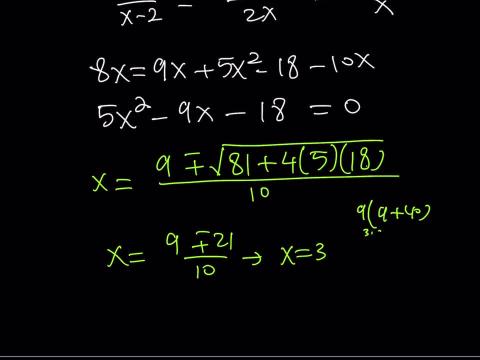 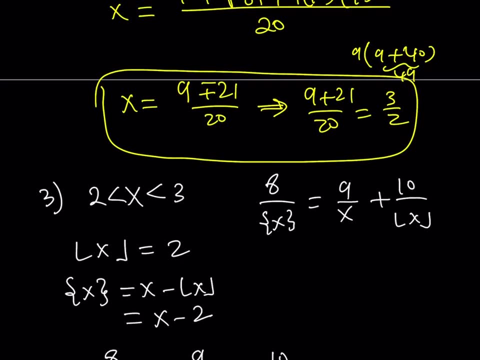 the equation, because when we plug it in, it just doesn't work, because it doesn't satisfy the inequality that we received. Okay, so we're not going to accept the solution, which means that the only solution in this case is going to be: x equals 3 halves. 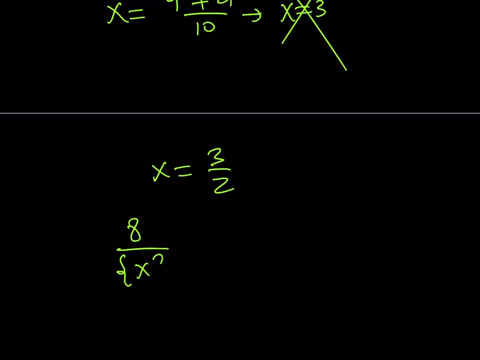 and our original equation one more time: 8 divided by the fractional part of x is equal to 9 over x plus 10 over floor value of x. Okay, and this brings us to the end of this video. Thank you for watching. I hope you enjoyed the video. Please comment, like and subscribe, and don't forget to 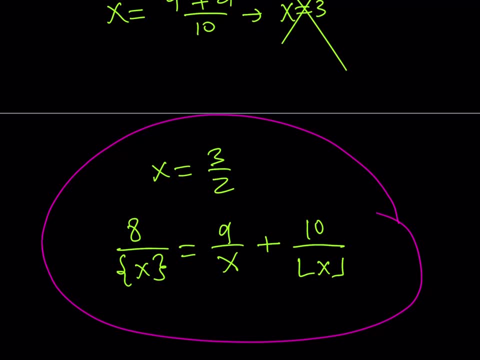 check out the merch. I'll see you tomorrow with another video. Until then, be safe and take care.